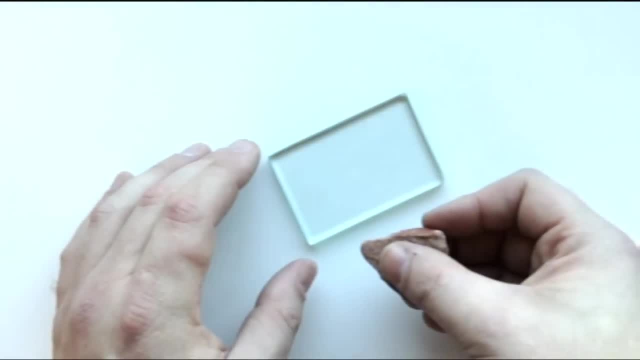 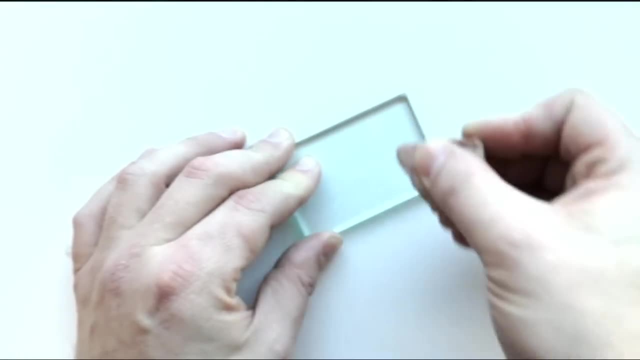 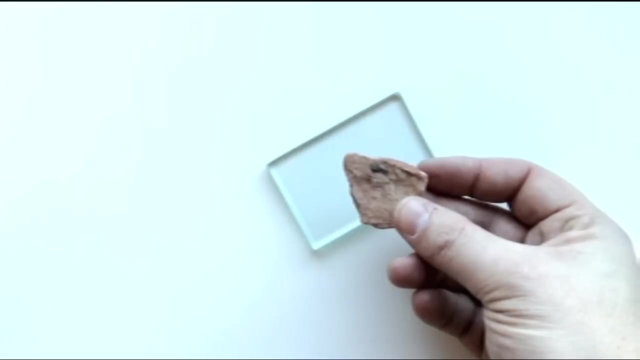 the surface, but you're also trying to listen and feel the glass. So I'm going to take a piece of glass to see if the sample is grinding into the glass or not. If it does scratch the glass, then this mineral has a hardness greater than 5.5.. If it does not scratch the glass, then it's less than. 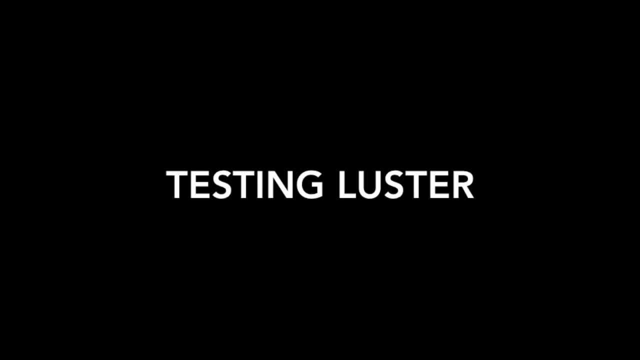 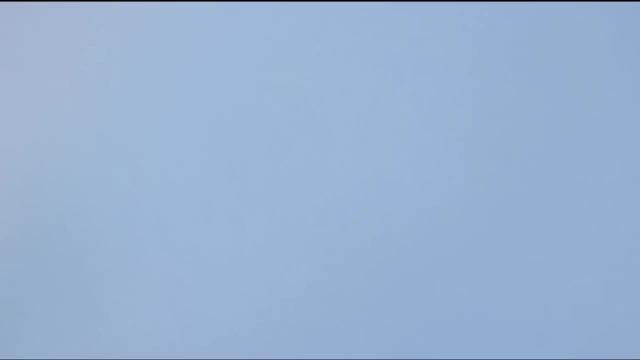 5.5.. Luster refers to how light reflects off of the surface of a mineral. For our class, we will be using two types of luster: Metallic and nonmetallic. Metallic minerals have a metallic appearance, And what I mean is that they are gold or 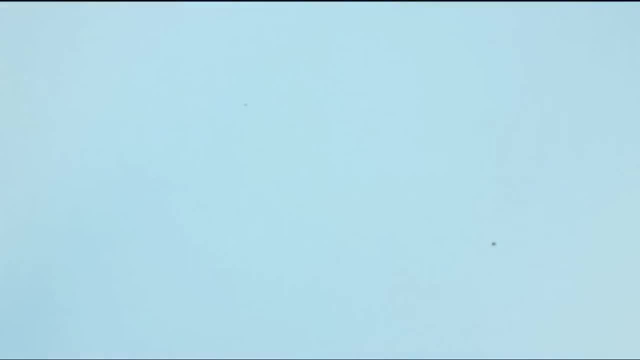 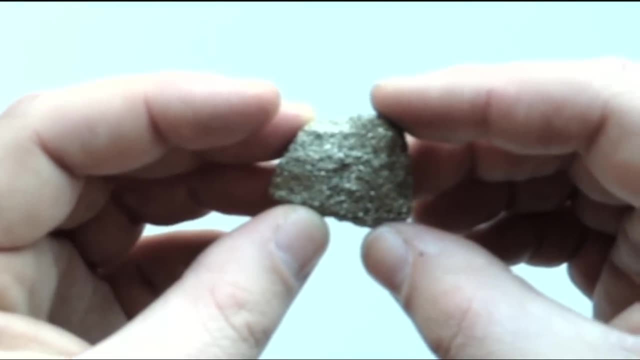 silver and actually look like a piece of metal, Like this chunk of galena or this chunk of pyrite. notice how they look like they're metal. So those have a metallic luster. So then there are other minerals like this. 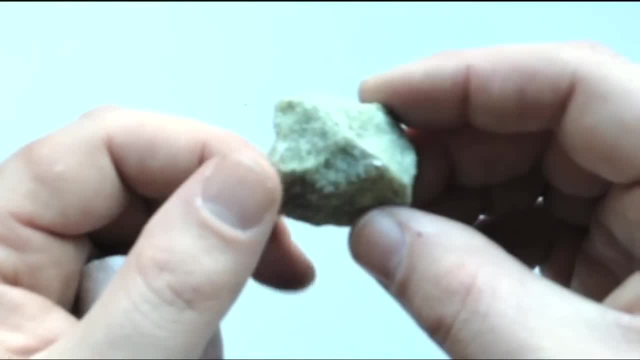 olivine, which does not look like metal And this has a nonmetallic appearance. And there are other minerals. these paper particles can be acáhol style, which is fine, But also a load surface is beautiful, although they are not sagen. 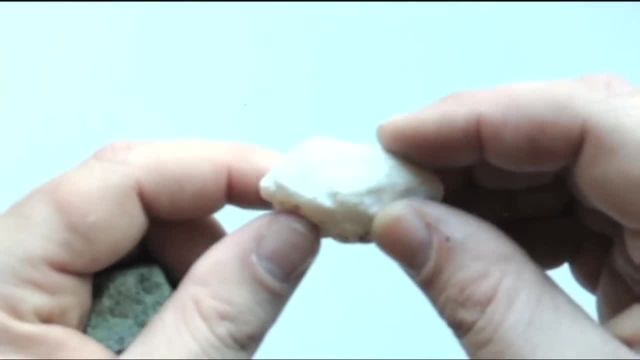 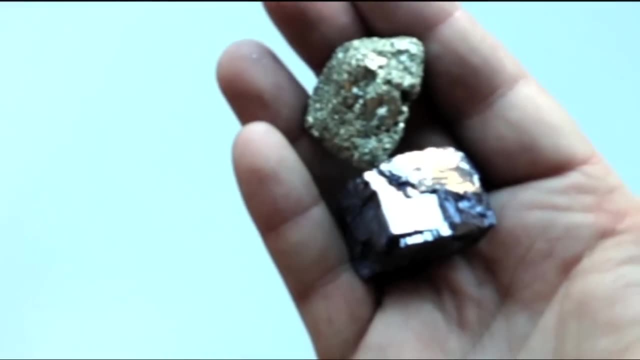 metallic luster, as does this gypsum. It does not look like metal. So when you're doing a luster test, all you have to do is ask yourself: do the samples look like metal? If so, they are metallic. Or do they not look like metal? If so, they are non-metallic. 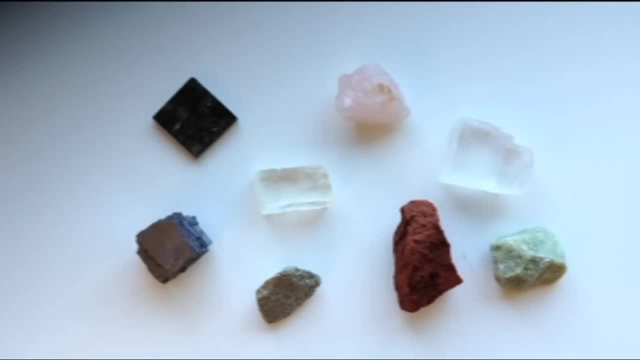 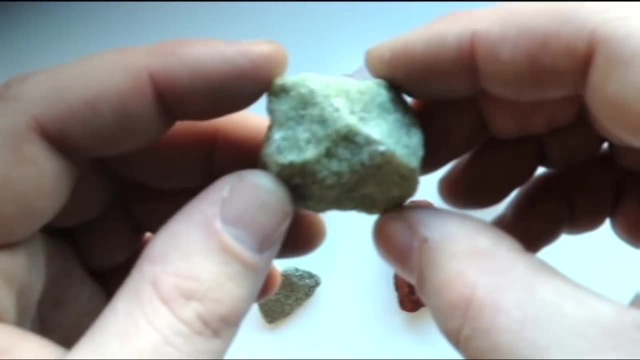 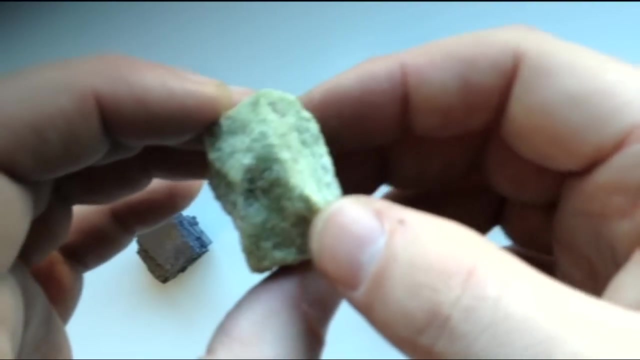 Breakage is probably the hardest property to identify. Minerals break in one of two ways: Cleavage or fracture. Fracture is when a mineral breaks randomly. If you look at this piece of olivine, you'll notice it has a jagged, irregular shape. It looks like it was just smashed into a 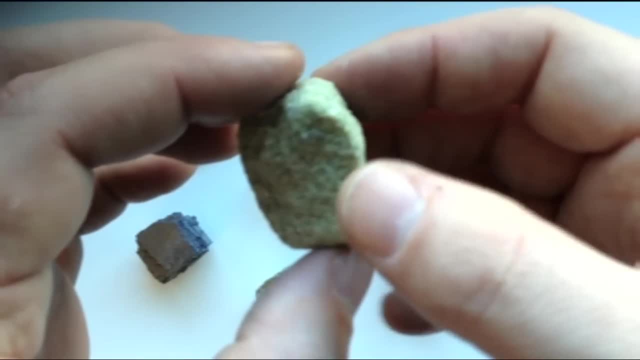 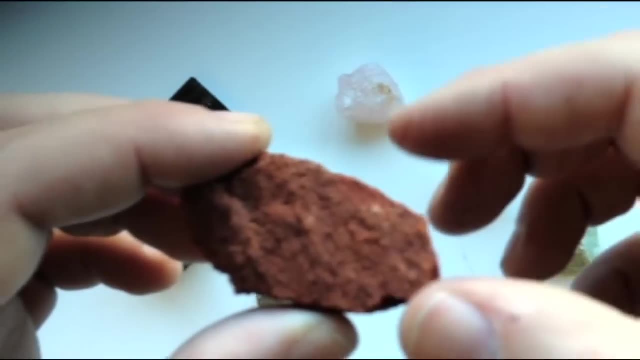 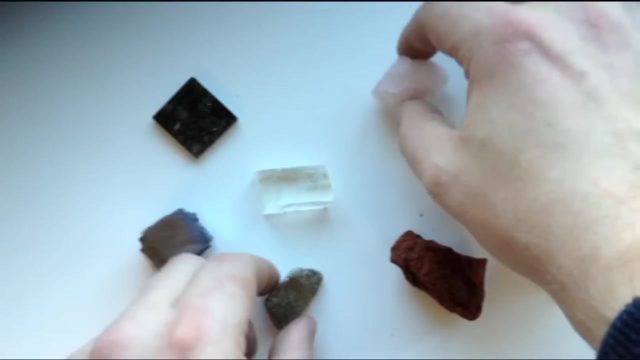 random shape. This is referred to as fracture. This mineral displays fracture. This red hematite also displays fracture. You notice the random irregular shape, As does this quartz sample- random and irregular, And this is the random irregular shape, And this is the random irregular shape. And this is the random irregular shape And this is the 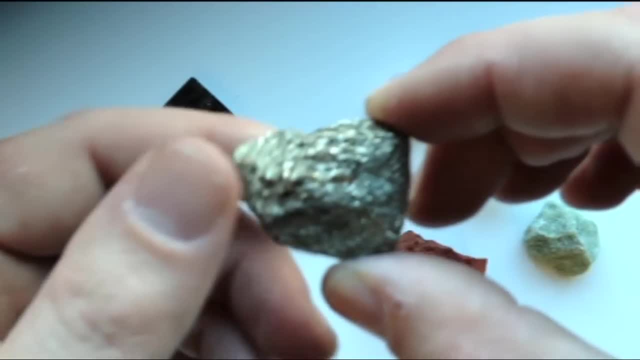 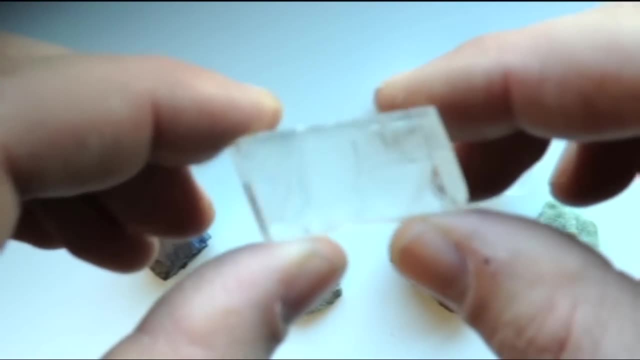 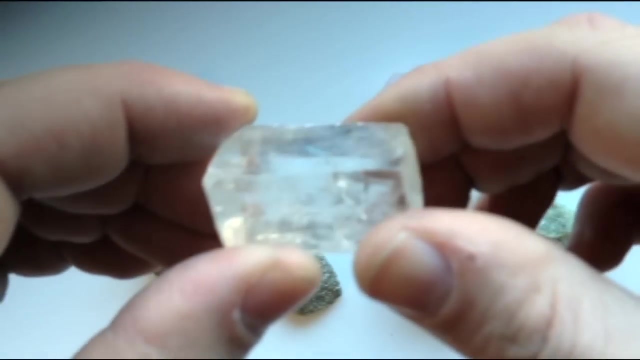 pyrite sample, random and irregular. That is fracture. However, there are some minerals on earth that break in very unique and predictable ways, like this piece of calcite. It almost looks like it was cut this way with a saw, But in fact this is the natural way that calcite breaks. 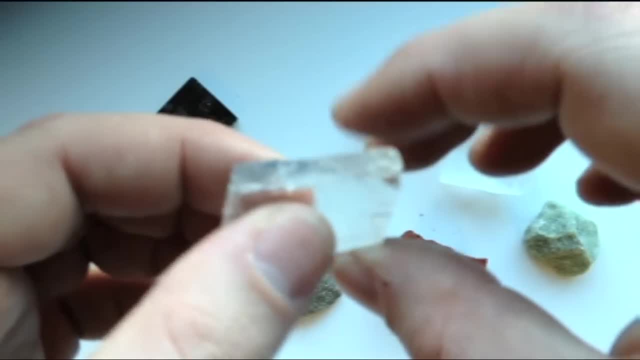 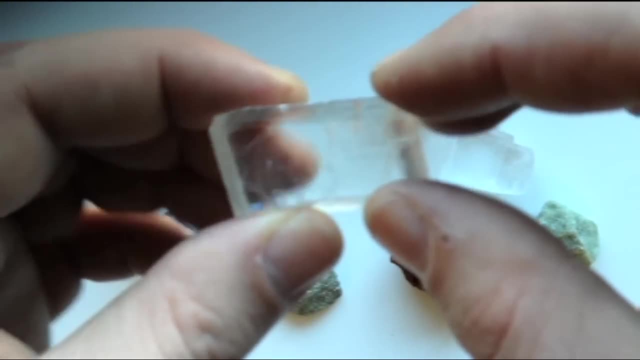 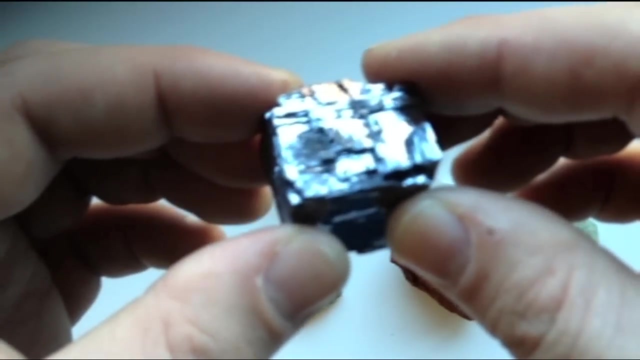 This breakage is referred to as cleavage. You'll notice it has predictable flat sides And if I were to smash this with a hammer, the little pieces that it created would be shaped similarly. This piece of galena has a really interesting type of cleavage If you look at it. 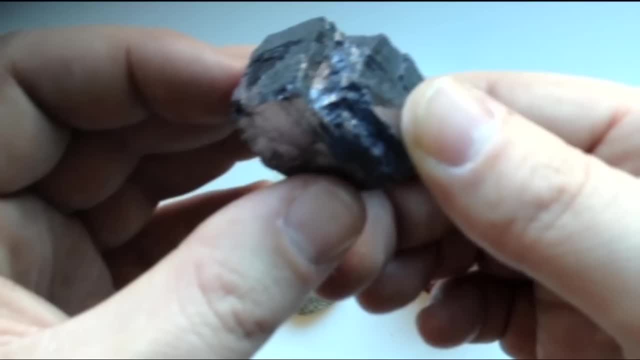 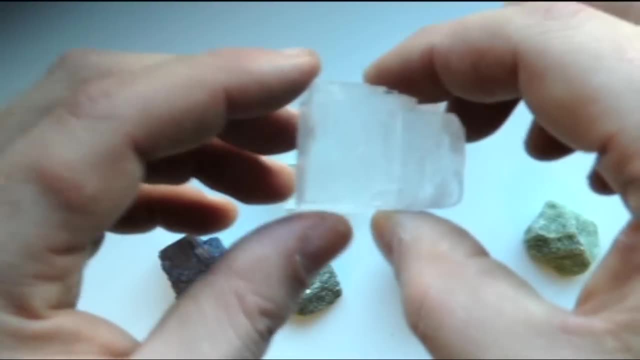 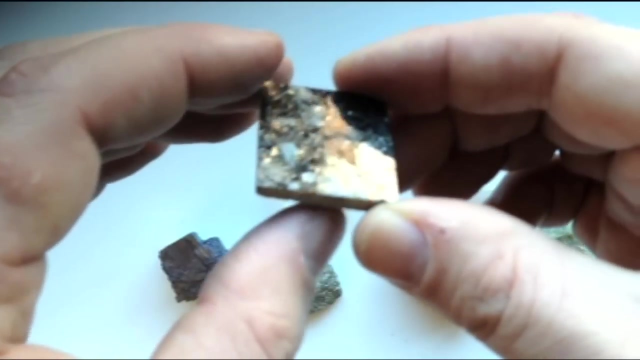 carefully, you'll notice that it, too, breaks at these predictable 90 degree angles, Flat sides. This was not cut this way. This is how it naturally breaks, As does this halite. This displays cleavage. There are some other types of cleavage as well. This is called biotite mica And it looks like a. 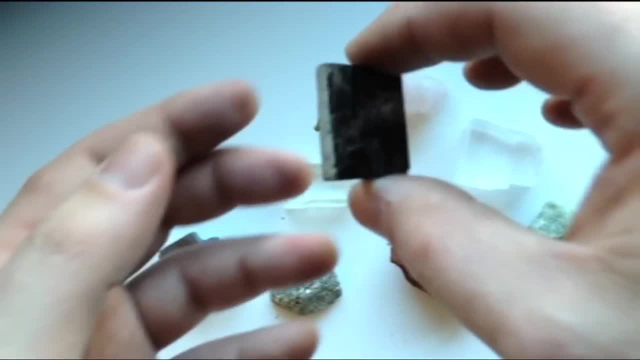 pyrite sample. But biotite mica is actually a type of cleavage, And what I mean by biotite mica is you can actually peel off thin pieces of it, And that is a different type of cleavage. I have a piece of 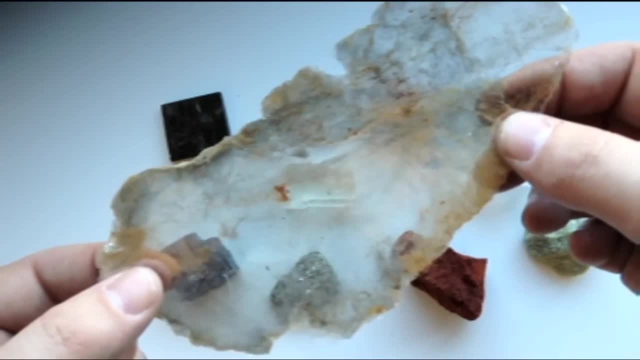 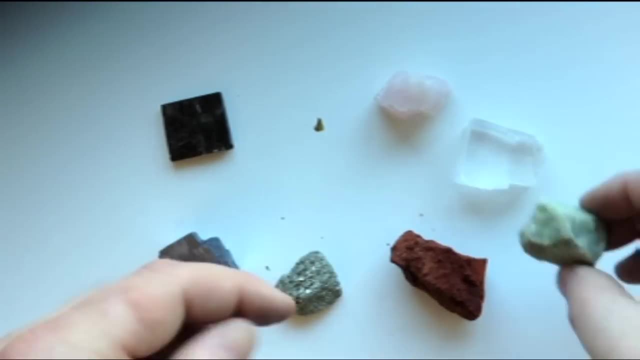 peeled off biotite mica. here You notice it's paper thin. This was peeled off of a larger sample. So just to sum up, cleavage is predictable. breaking like this calcite Fracture is random. breaking like this olivine. Streak refers to the color of a mineral And this is the color of a mineral, And this is the color of an mineral, And this is the color of a mineral, And this is the color of a mineral, And this is the color of an. 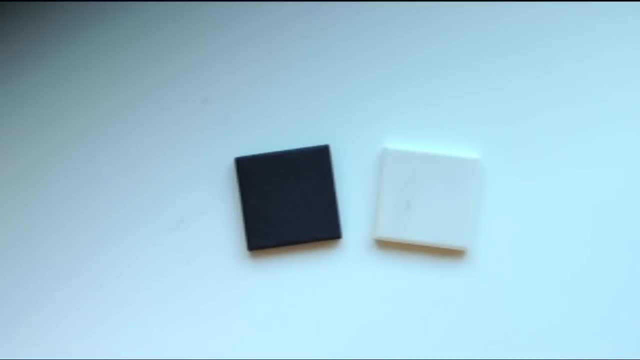 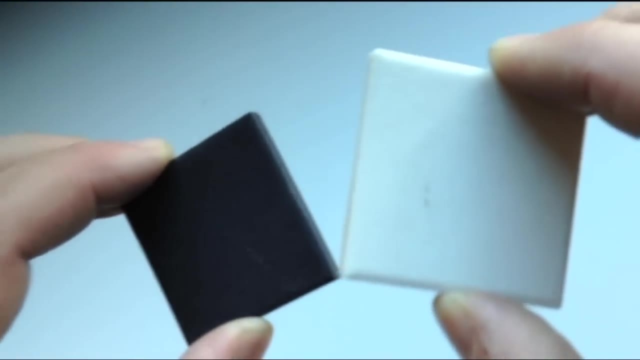 mineral as a powder. In order to make a powdered sample of a mineral, we use streak plates. These are ceramic tiles. One is black and one is white, And what we do is we place them on the desk and we rub our mineral samples against them to create some powder and see. 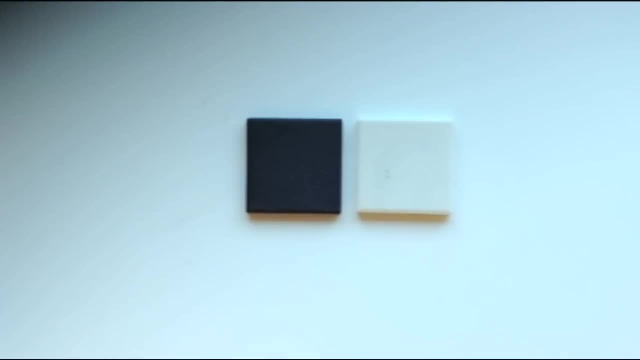 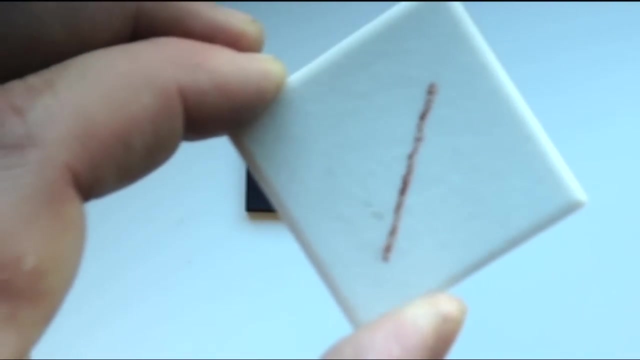 what color that powder is. Let me demonstrate. This is a piece of red hematite. I'm going to take this hematite and I'm going to gently, one time, try and draw a line And what you notice is that it has a reddish brown streak. I would refer to that as a colored streak. 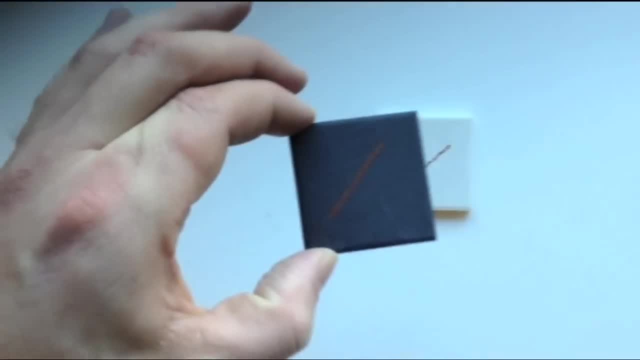 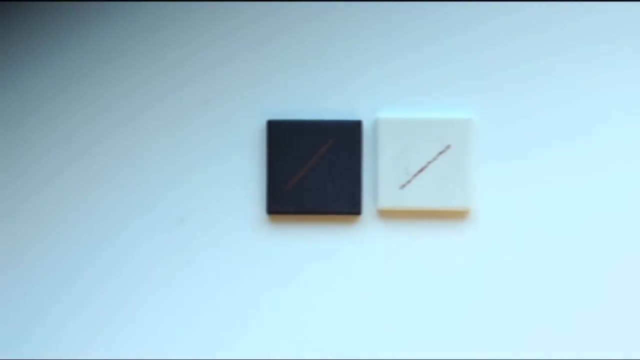 If I try it on the dark plate I will see it and I can more clearly see the color. So when we do streak tests, we often try it on both the black plate and the white plate. Let me give you another example. This is pyrite- Notice how it looks gold. But when I powder,